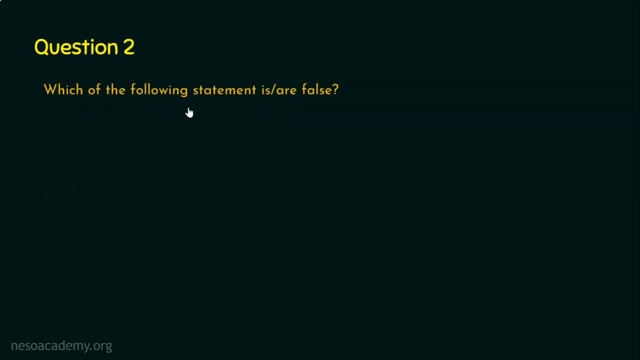 to question number two. The question is which of the following statement is, or are false Options are: option A: both file system and database management system are preferred for storing and retrieving the data. Option B: file systems can handle redundancy well. Option C: database systems are more responsive data. 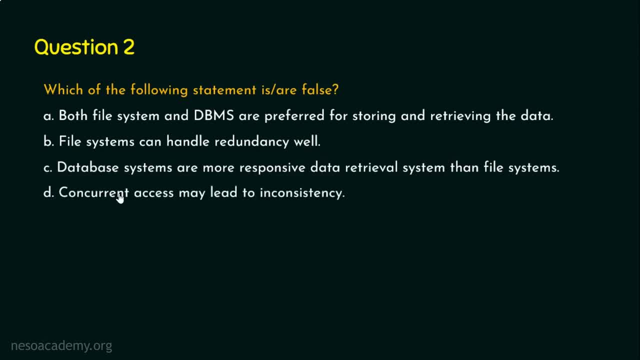 retrieval system than file systems, And option D, concurrent access, may lead to inconsistency. I request you to pause this video for a while and think about the right answer. I hope you are done. In this question, we are required to find out the false statements. 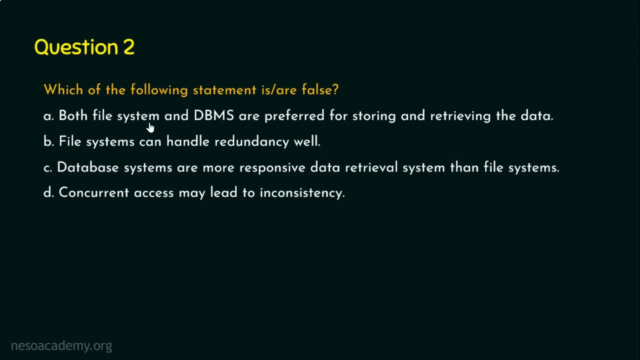 At first we will focus on the first option. both file systems and database management system are preferred for storing and retrieving the data. This is true because both file system and DBMS are for storing and retrieving the data only. But the difference is file system is not efficient in terms of effective storing and retrieval of data, Whereas 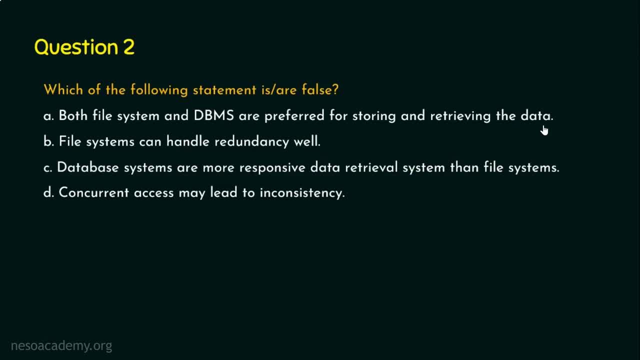 DBMS is efficient, But anyway, both file system and database systems are for storing and retrieving the data, So this is not the right answer. So A is not the right answer. Coming to B, file systems can handle redundancy well, And this is false, And this is one of the drawbacks that we have in file. 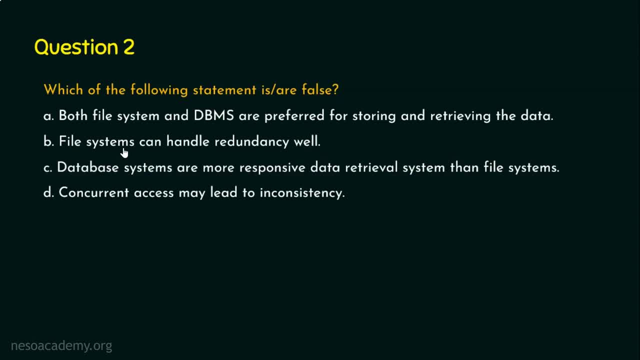 systems And that is why we are preferring DBMS. So option B is false. So we can confirm that one of the right answers here is: file systems can handle redundancy well, which is actually not true. Let's see. is there any other correct answer? Database systems are more responsive data retrieval. 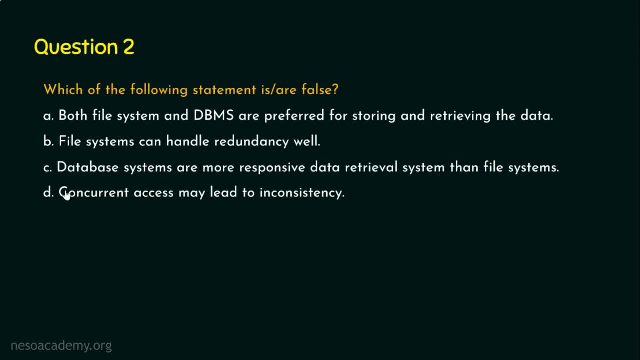 system than file systems, And this is also true. And coming to option D, concurrent access may lead to inconsistency. This is also true, But concurrent access in databases are handled well. But anyway, in general concurrent access may lead to inconsistency if it is not properly handled. So from this we can 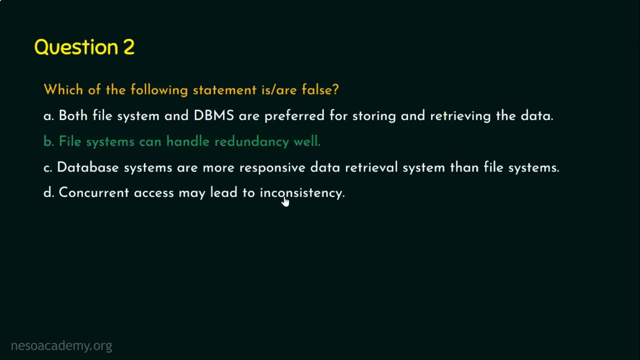 confirm that the right answer is option B, that is, file systems can handle redundancy well, which is false. We are done with question number two. Let's now move on to question number three, which is in the following tier, deals with the business logic and business rules, And the options are given. 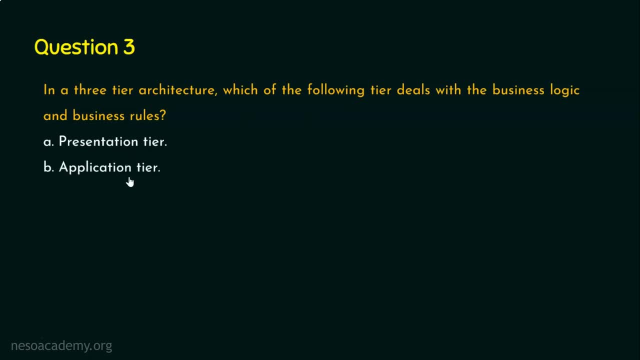 option A- presentation tier. option B- application tier. option C- data tier. and option D: none of the above. I request you to pause this video for a while and think about the right answer. I hope you are done. Let's analyze what's the question In a three-tier architecture. 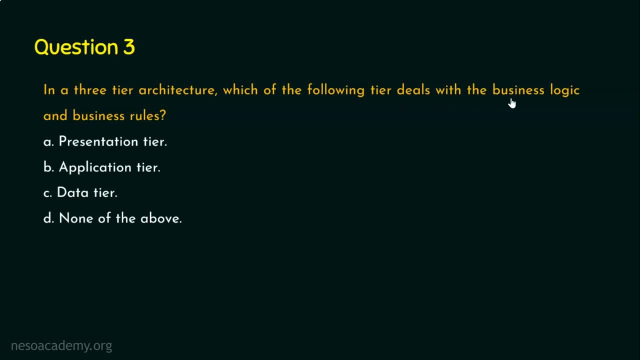 we are required to find the following tier that deals with the business logic and business rules. Presentation tier is the front end, So this is not dealing with the business logic and business rules. Its intention is to provide interface to the user to access the 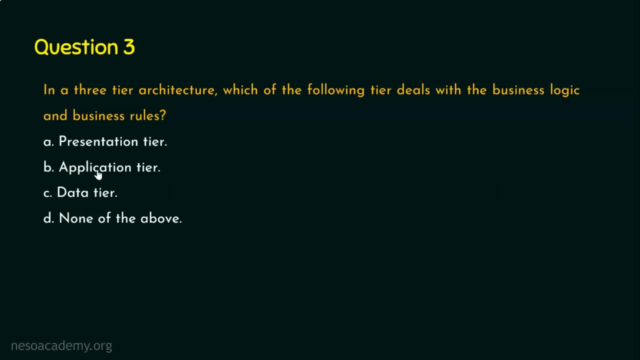 database And application tier. yes, this is the tier that deals with the business logic and business rules. And coming to the data tier, we have databases here, which does not deal with the business logic or business rules, And hence option B is the right answer here. 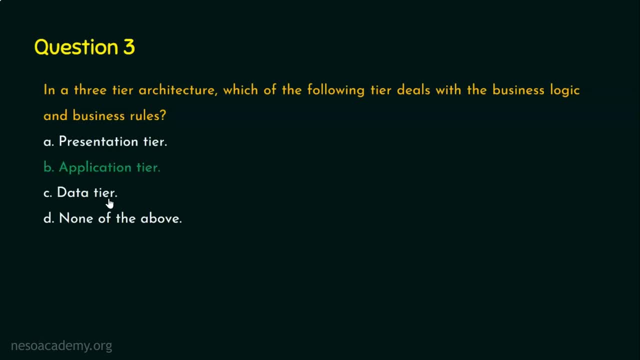 We are done with question number three. Let's now move on to question number four. The question is hiding the complexity from the application programmers and users is referred to as dash, And the options are: option A- data encapsulation, option B- data redundancy, option C- data abstraction and option D- data analytics. 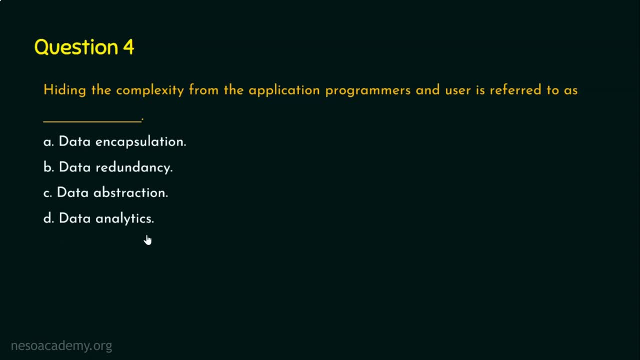 I request you to pause this video for a while and think about the right answer. It's easy to answer this question: that data abstraction is the right answer, because data is the concept that hides the complexity from the application programmers and also from the users accessing the database systems. So we want simplicity. We don't want any complex details. 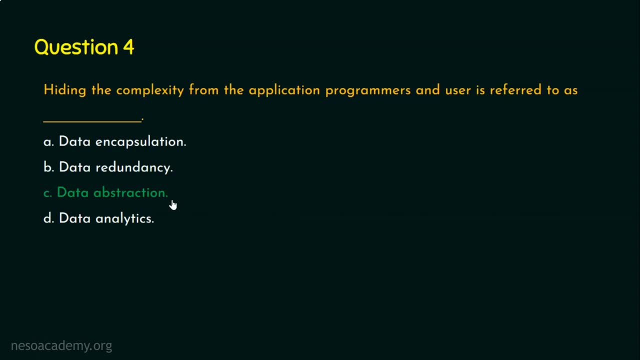 to be shown. So we are hiding the complexity through data abstraction. We are done with question number 4.. Let's now move on to question number 5, which is the overall design of the database, is called as dash, and the options are: option A- schema, option B- instance, option C. 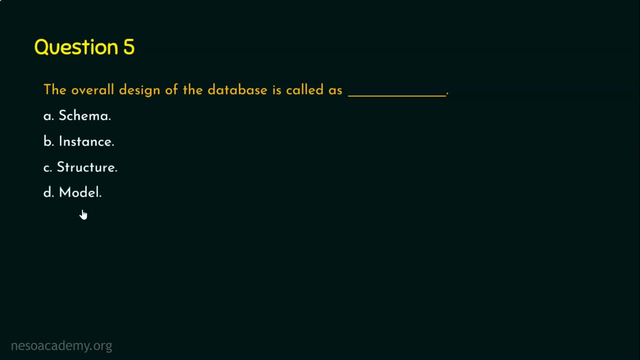 structure and option D model, and we can confirm that the right answer for this question is option B schema, because schema is referred to as the overall design of the database and we have three levels of schema: The physical schema, the logical schema and the sub schema. We are done with. 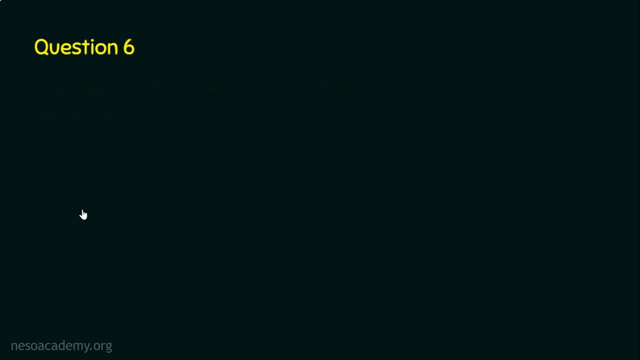 question number 5.. Let's now move on to question number 6.. The question is which of the following type of users are unsophisticated and who interact with the system by invoking one of the application programs that have been written previously, and the options are: 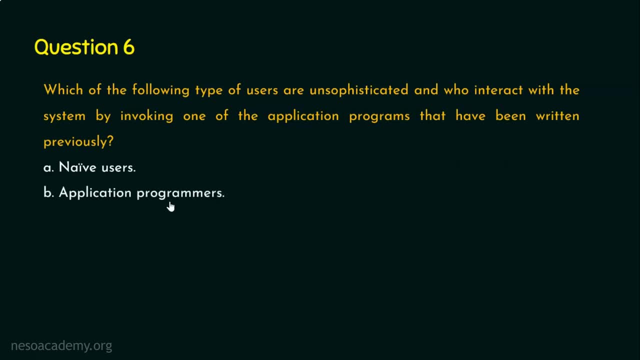 option A- naive users. option B- application programmers. option C- database administrators. and option D- system analyst. I request you to pause this video for a while and think about the right answer. I hope you are done, and the right answer for this question is option B- schema. 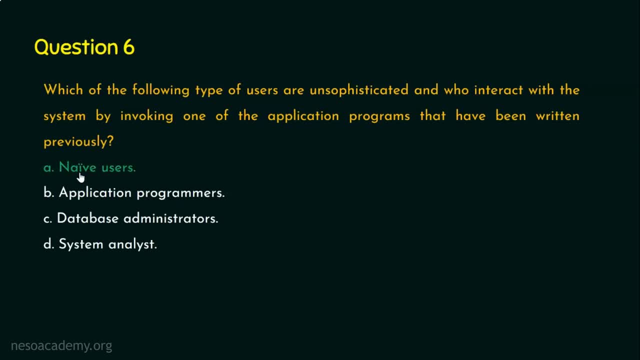 So this question is option A- naive users- because naive users are the unsophisticated users who interact with the database system by invoking the application programs that were written by the application programmers and also coming to the database administrators. they have the overall control over the system and they are not unsophisticated users Coming to the system. 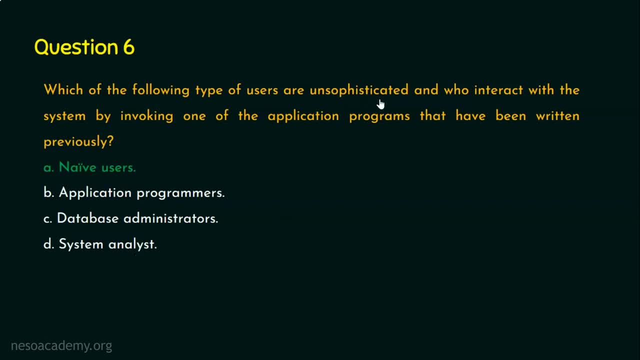 analyst or database analyst. he is also not an unsophisticated users. So the unsophisticated here, who invokes the application system, is the unsophisticated users. So the unsophisticated application program is the naive users, Tellers in the bank, even end users who access the database. 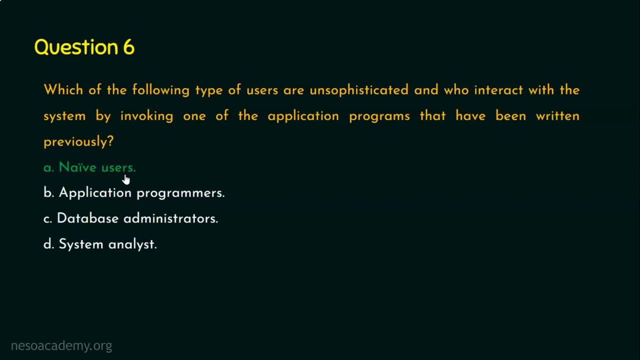 system through some web interfaces are referred as naive users. We are done with question number six. Let's now move on to question number seven, and the question is which of the following is, or are incorrect about DBA, the database administrator? The options are: DBA is responsible for granting. 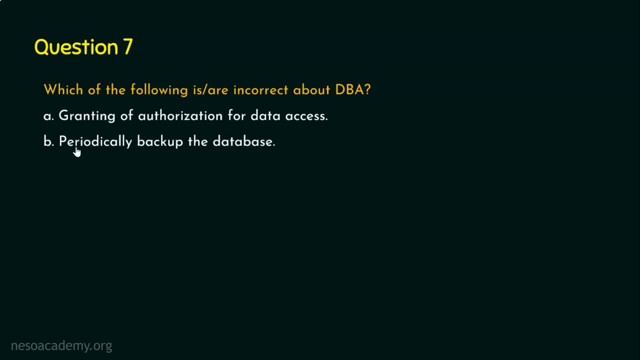 authorization for data access. Option B- DBA- periodization: periodically back up the database. Option C: DBA- defines the DBA schema storage structure and the access method. and option D: None of the DBA regime. I request you to pause this video. 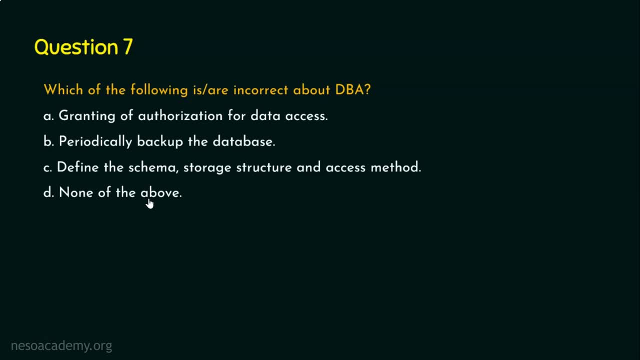 for a while and I think about the right answer. Option D: None of the above. because of all these jobs mentioned, Option A and B are all the responsibilities of the database administrator and hence option D N is the correct answer. Here is the correct answer. 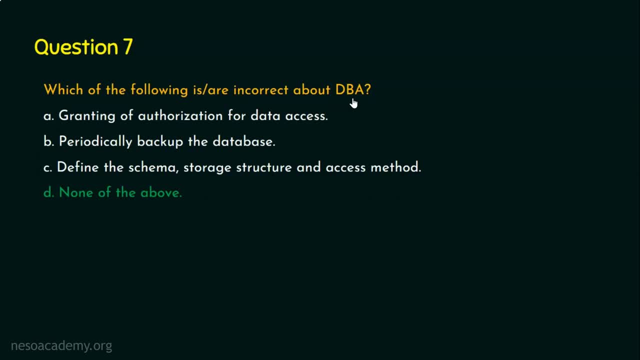 Let's go and see which of the options are correct. Page number to So DBA: the database administrator grants the authorization for data access, periodically backup the database and he is the one who defines the schema storage structure. and.